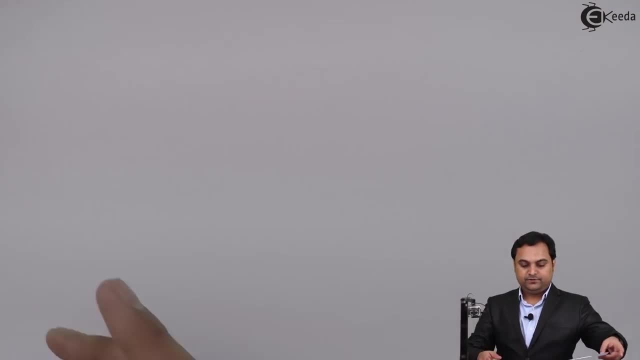 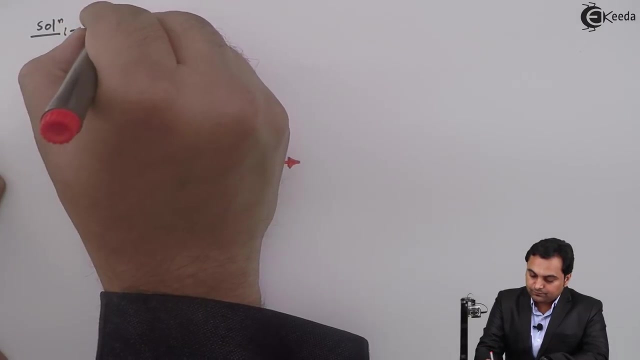 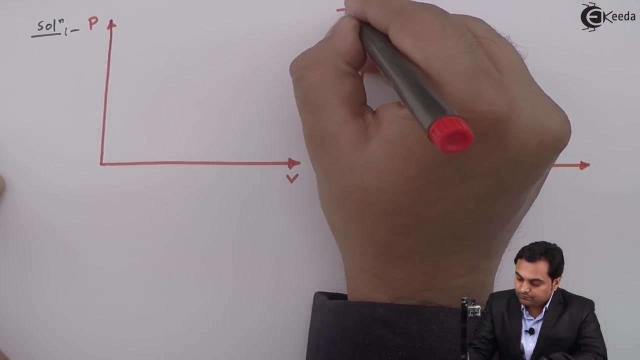 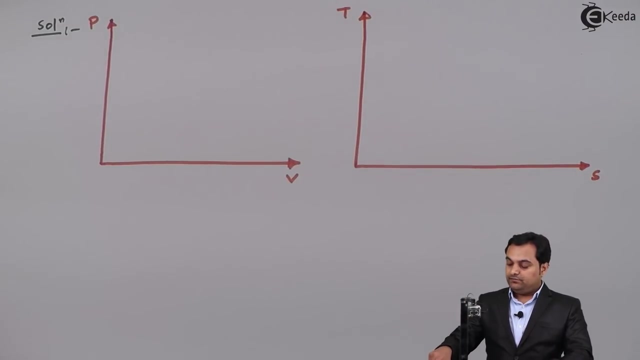 Now in the solution part, since the problem is on Carnot cycle, we first need to draw the Carnot cycle on PV and T-S diagram. Now in Carnot cycle, the first process is isentropic compression and that can be shown. 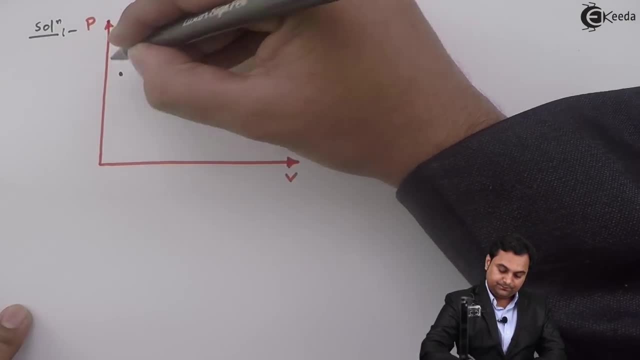 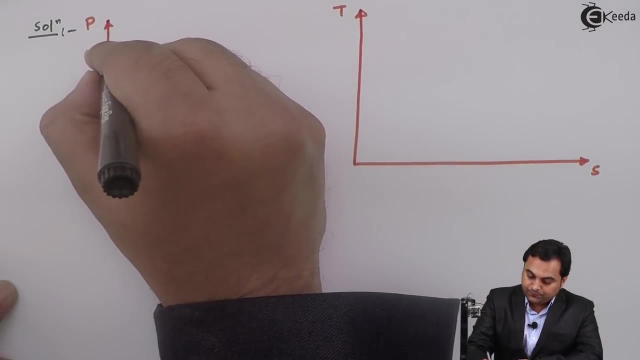 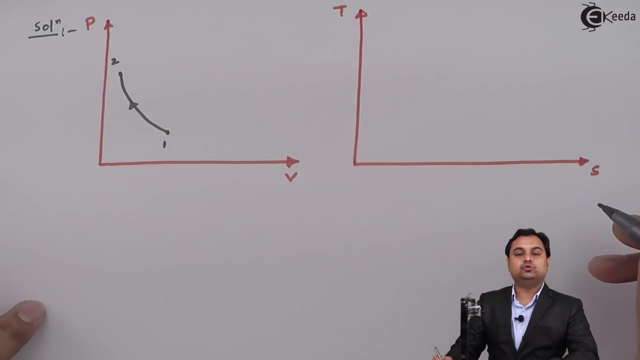 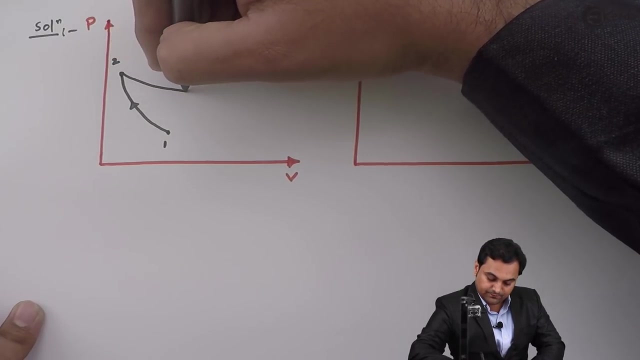 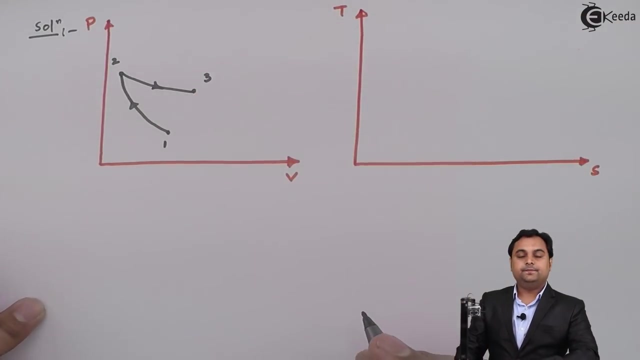 on the PV diagram with the help of a curve. So here we have process 1 to 2 as isentropic compression. Next, process 2 to 3 is isothermal heat addition. So again, isothermal lines on PV diagram. it will be a curve from 2 to 3.. 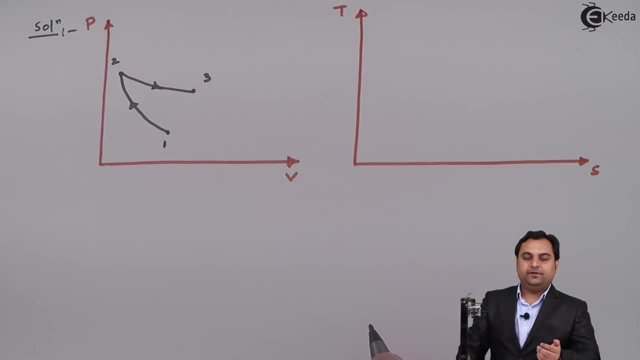 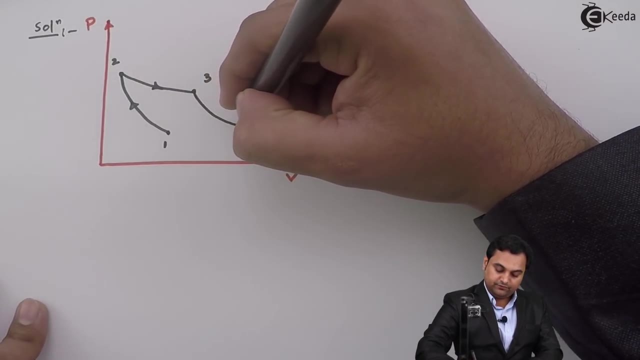 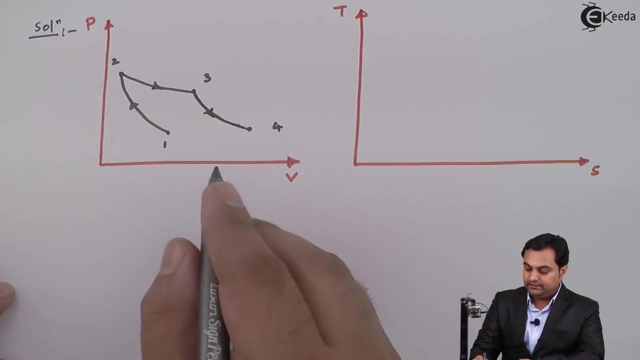 Then the next process, 3 to 4, is isentropic expansion. like here, it was isentropic compression, now we have isentropic expansion again, following a curve from 3 to 4.. And at last we have the heat rejection process, which is again at isothermal heat rejection process. that 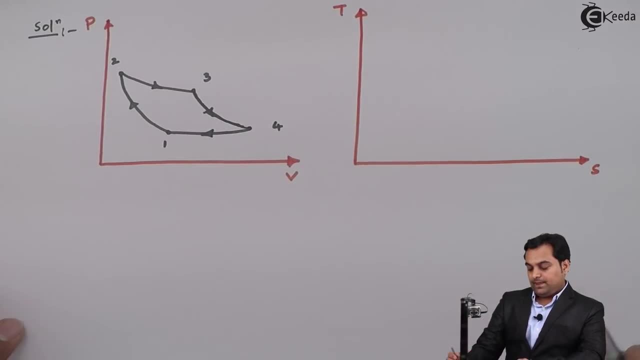 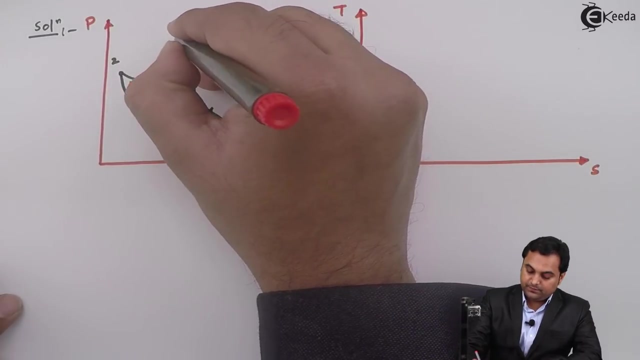 is at constant temperature. So here I have drawn the PV diagram for Carnot cycle And next I can draw it on TS diagram as well. The first process is isentropic compression. So isentropic compression is governed by the law. PV raised to gamma is equal to constant. 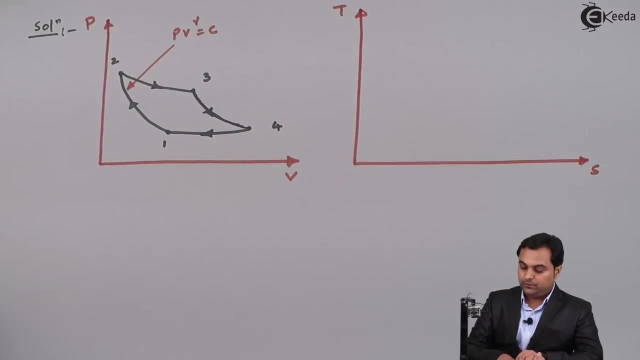 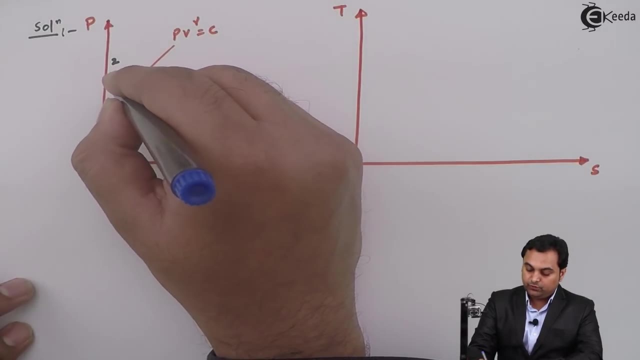 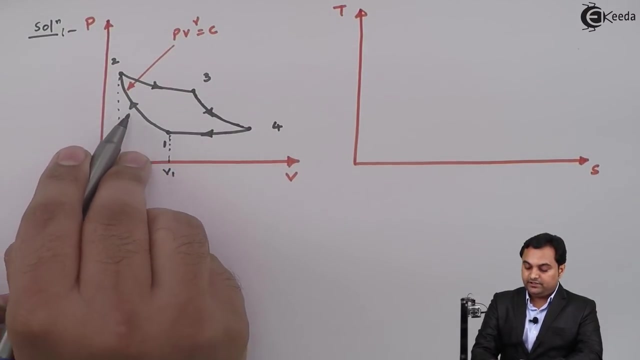 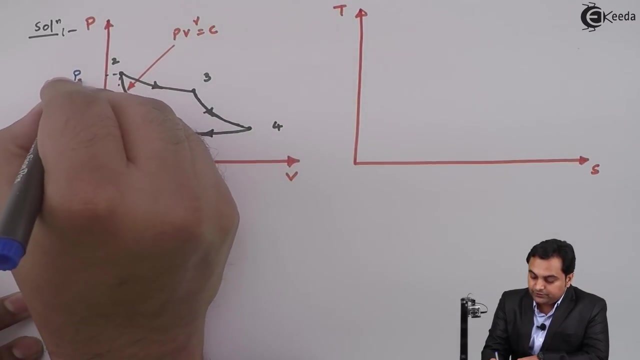 And it means that the entropy remains constant during 1 to 2 and, as we see, at point number 1 the volume is more, at point 2 the volume is less. So by the reduction in volume we are getting the increase in pressure, that is, pressure increases from point 1 to point 2.. 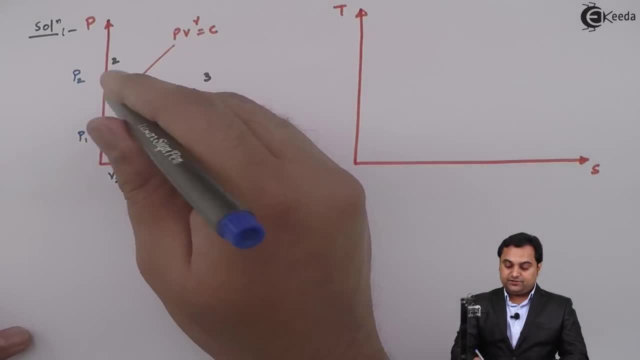 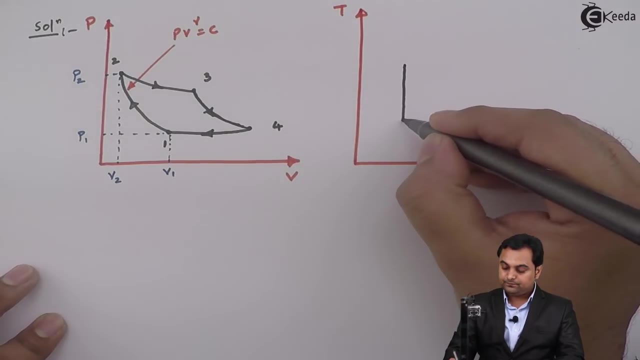 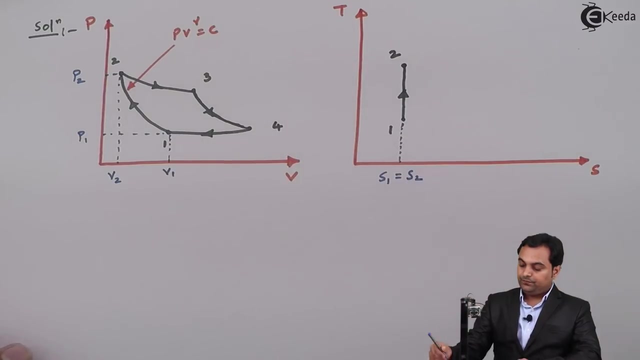 So here this is isentropic compression. it can be shown on the T-S diagram with the help of a vertical line. Process 1 to 2 is isentropic compression and entropy remains constant. So S1 is equal to S2.. Then process 2 to 3 is isothermal heat addition. 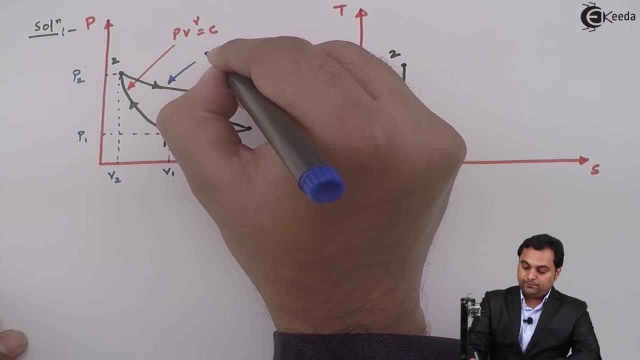 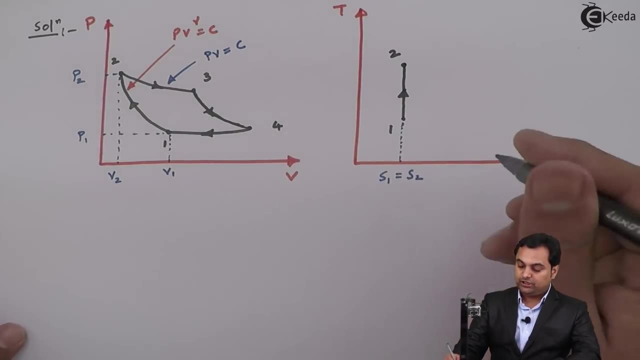 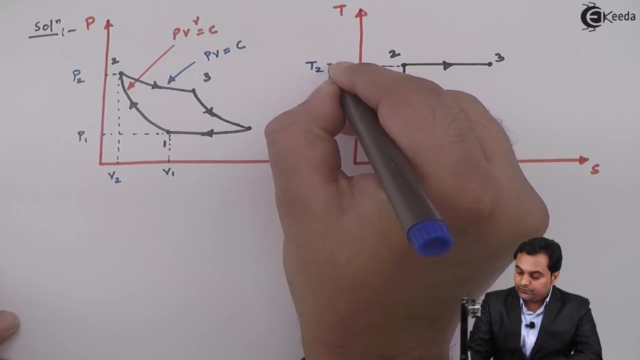 And isothermal lines. it follows the law. PV is equal to constant, that is, the temperature remains constant here. So this heat addition process is isothermal. so the temperature remains constant from point 2 to 3.. That is, T2 is equal to T3.. 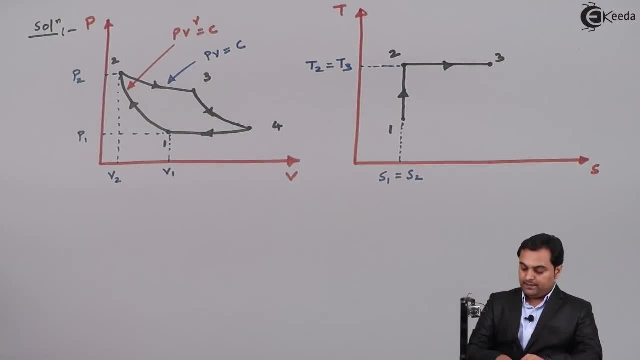 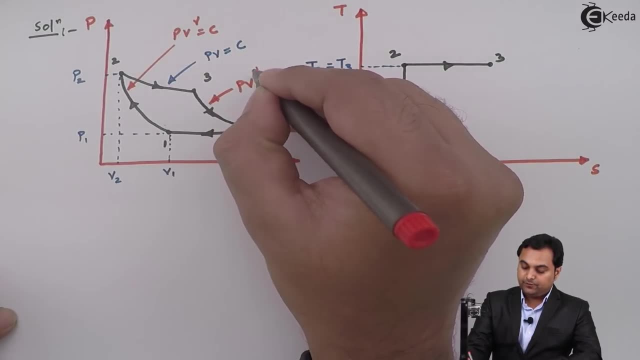 Then 3 to 3 is isothermal, Then 3 to 4 is again isentropic expansion, like here it was for 1 to 2 isentropic compression. For 3 to 4 it is isentropic expansion. PV is to gamma is equal to constant. 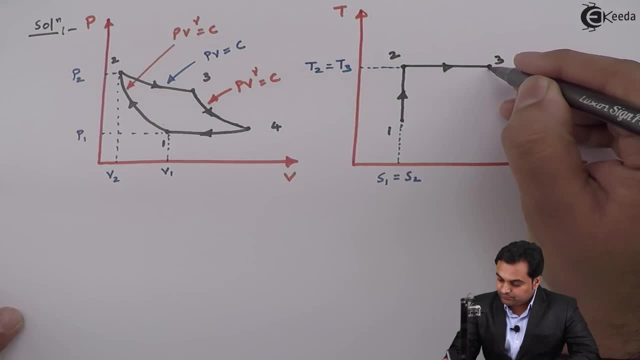 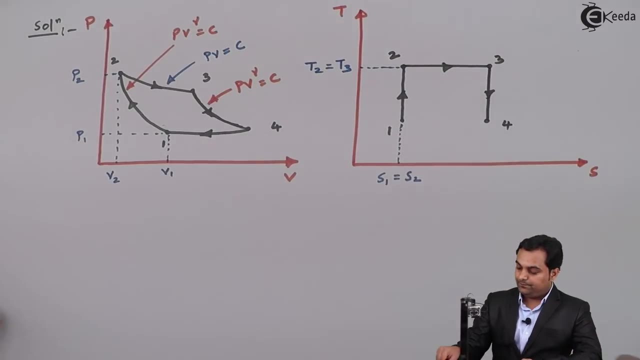 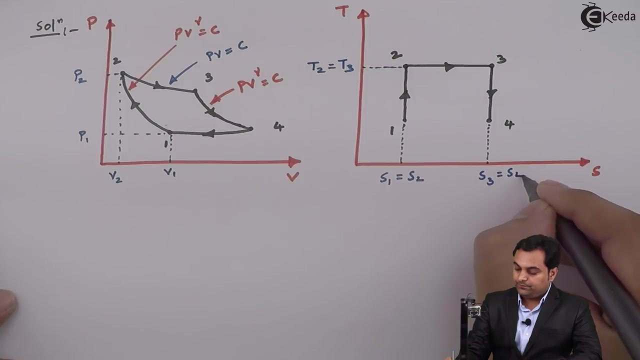 So again, isentropic expansion can be shown by a vertical line. So from 3 to 4 the entropy remains constant, S3 is equal to S4. And here we have the expansion process in which the entropy remains constant But there is drop in temperature from point 3 to point 4.. 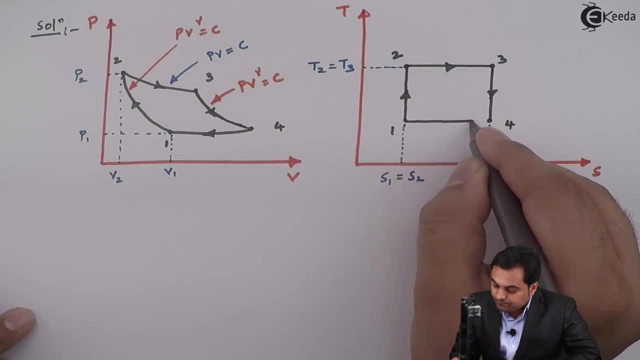 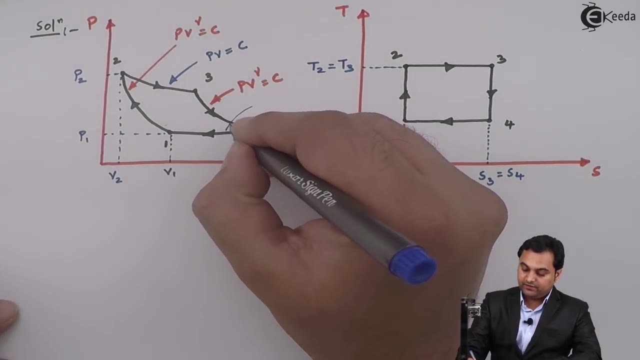 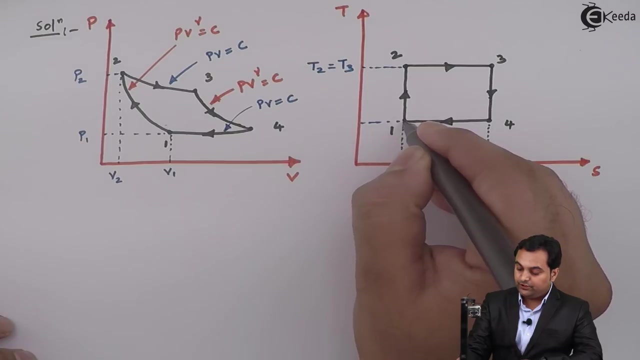 Next, from 4 to 1, it is the heat rejection process which is at constant temperature, or we can say isothermal heat rejection. PV is equal to constant. So here, as we see the temperature of point 1 and 4, they are same. 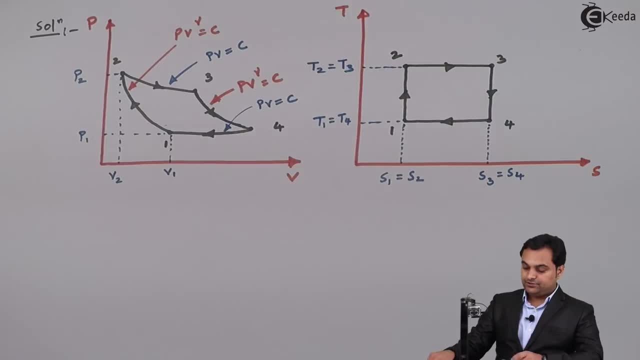 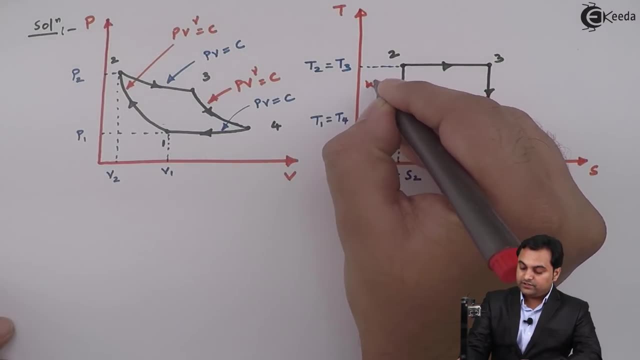 So T1 is equal to T4.. That is the heat rejection process. So I can mark all the processes on this diagram, That from 1 to 2 it is compression. So work is done on to the system during the compression process. 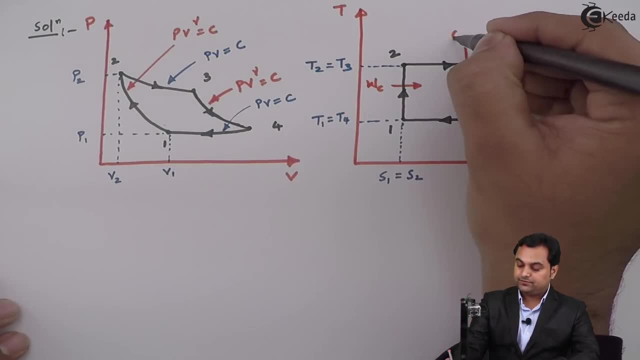 During 2 to 3 there is heat addition into the system, So Q suffix A. From 3 to 4 there is isentropic expansion. So work is done or we are getting the work output during expansion process And 4 to 1 is the heat rejection process. 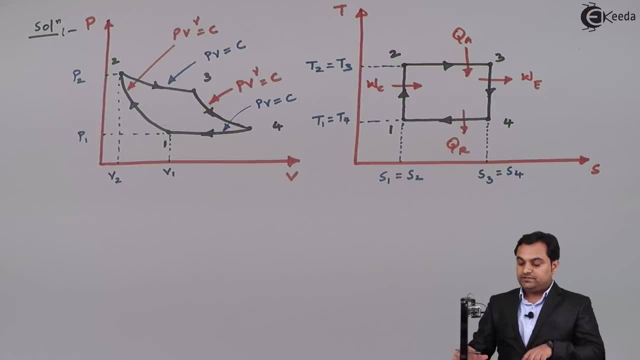 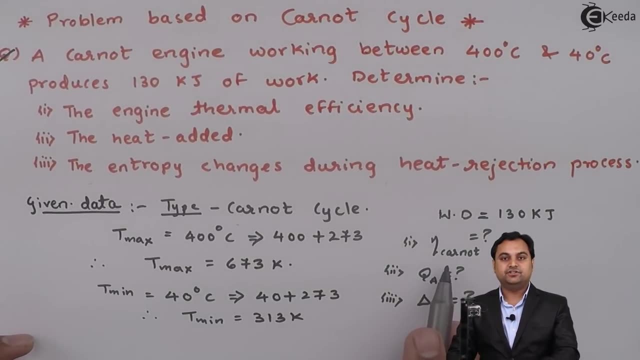 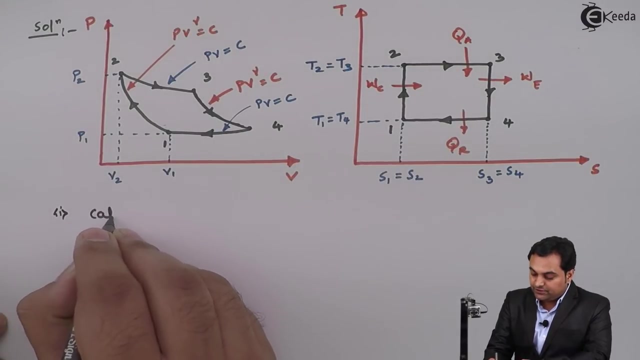 Which is Q suffix R. Now this is the Carnot cycle which we have. If we look at the question, the first thing is we have to find out Carnot efficiency. Now I will write down that the first thing is calculation of Carnot efficiency. 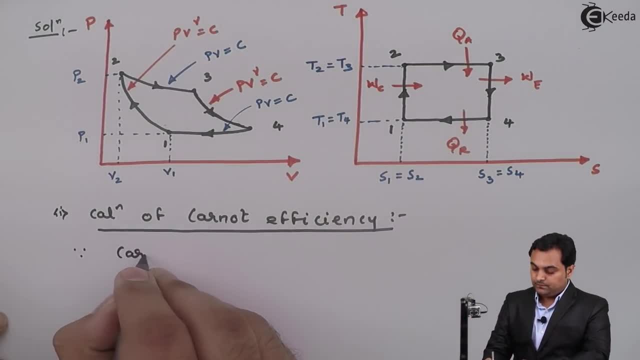 I will write down, Since Carnot efficiency is given by efficiency of Carnot engine is equal to maximum temperature minus minimum temperature upon maximum temperature And if we look into the diagram, I can say that T2 is the maximum temperature. It is equal to T3.. 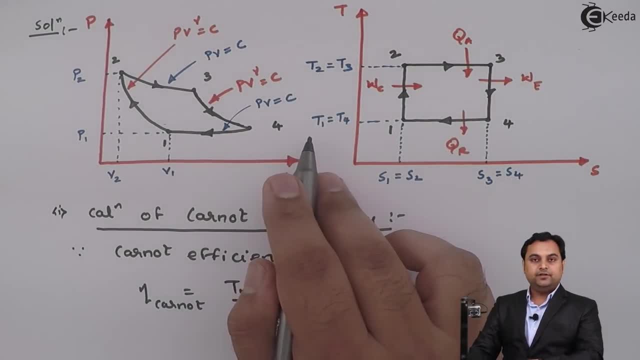 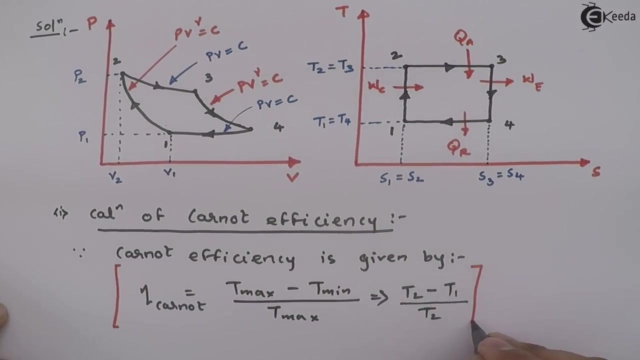 So we can write either T2 or T3. Then T1 is the minimum temperature, So minus T1. or even, if I want, I can write it as T4. Because both are same And Tmax is T2.. So here is the formula to calculate the efficiency of Carnot cycle. 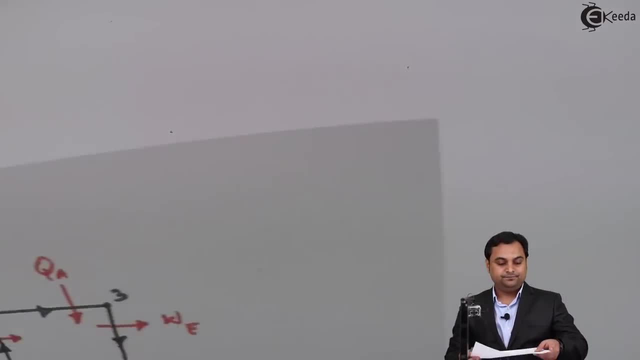 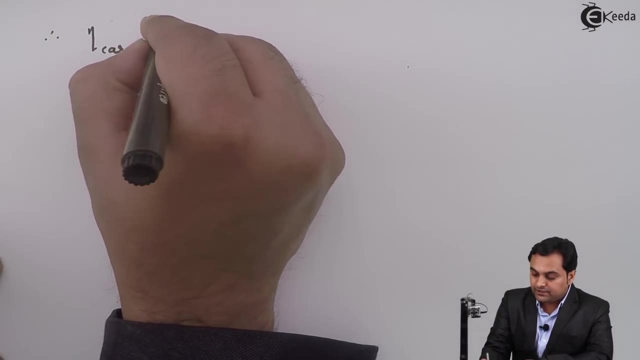 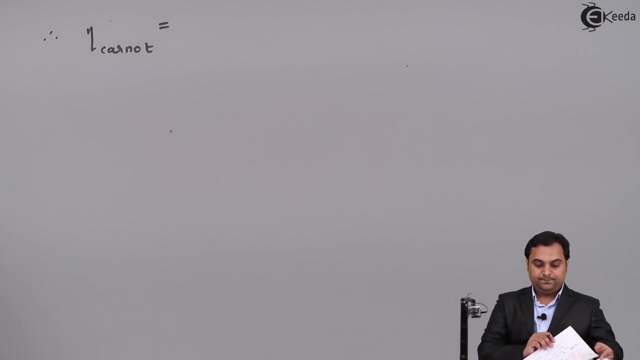 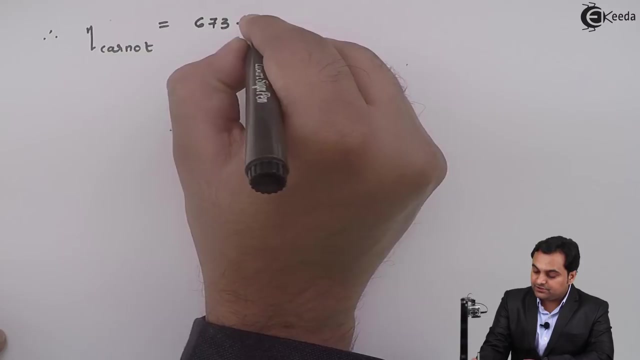 Next I will go on putting the values which are given in the problem. So therefore, Efficiency of Carnot cycle is equal to now the maximum temperature Tmax. It is given in the problem as 673 and Tmin is 313.. So I will put the values: that efficiency of Carnot cycle is maximum temperature 673, minus minimum temperature 313, divided by the maximum temperature which is 673.. 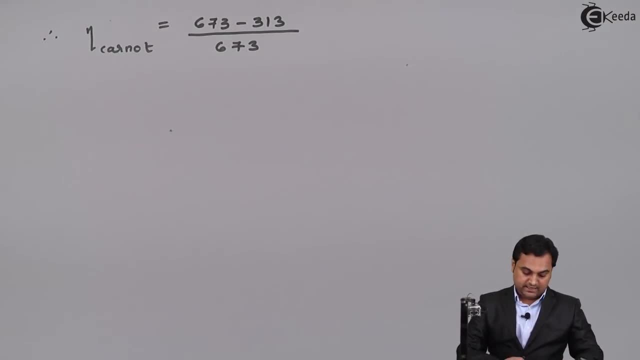 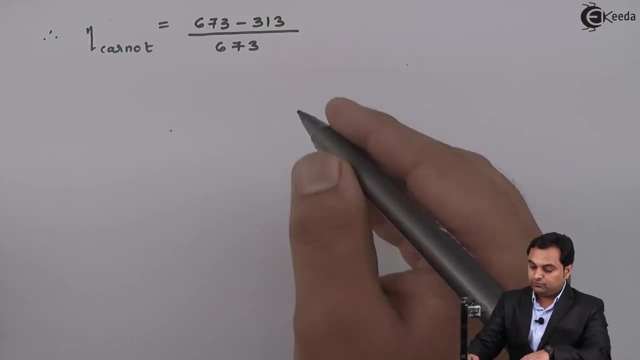 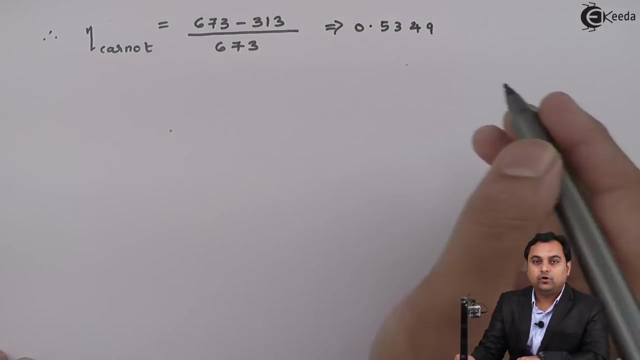 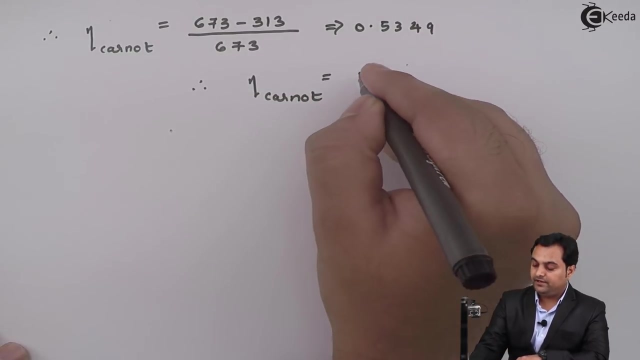 So after this, when I am calculating this, I will get my answer, as It comes out to be 0.5349, or therefore I can say that Carnot efficiency is equal to. I have to multiply it by 100.. So it becomes 53.49%. 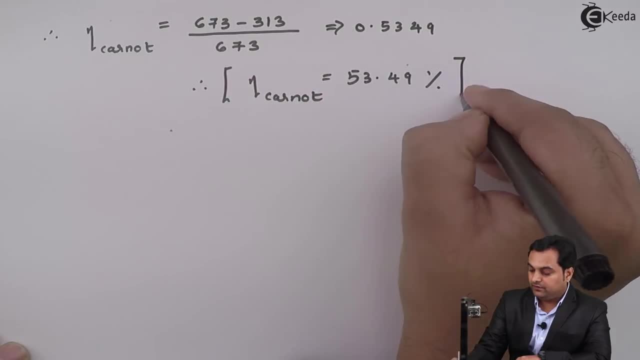 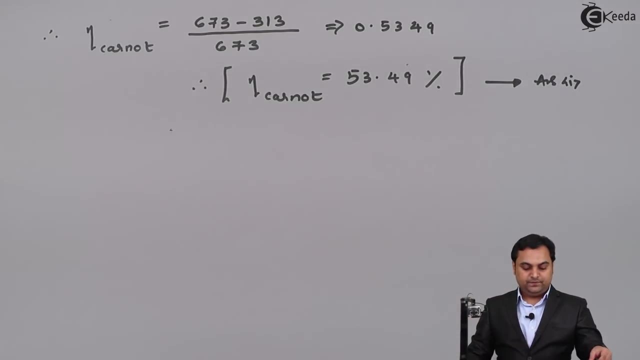 So this is the first answer for us. So now, once we have calculated the Carnot efficiency, The next thing is we have to find out how much is the heat added, That is, heat supplied during the isothermal heat addition process. So the next thing is: 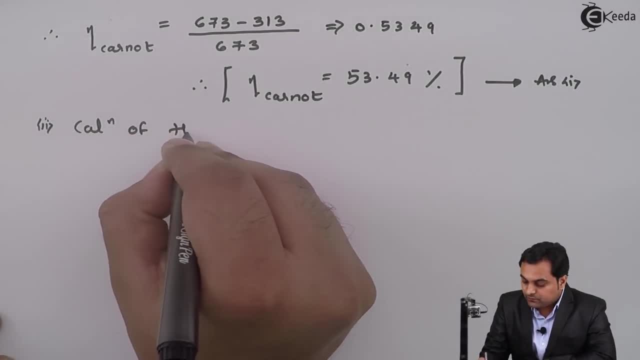 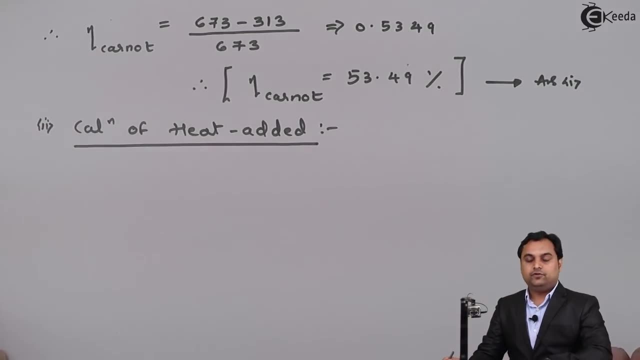 Calculation, Calculation of heat added. So for this again I am using the concept of Carnot efficiency. That, since efficiency of Carnot cycle, It can also be written, as As previously we have written that in the form of temperatures, Now I can write them in the form of output by input. 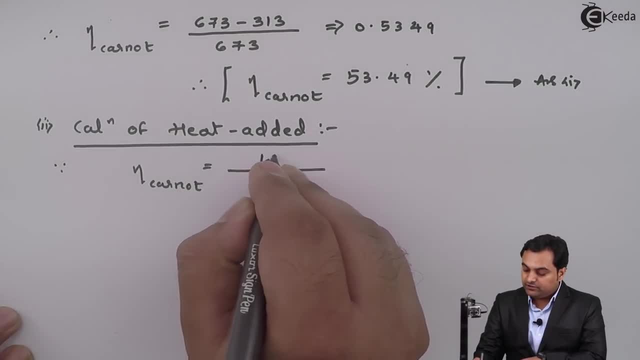 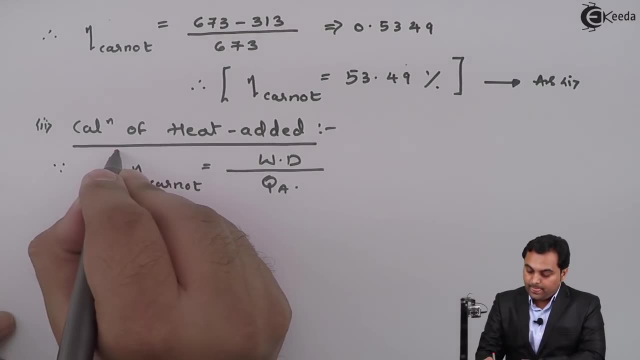 So output is the work which we are getting, That is the work done, And input is the heat which is added, So I can use this concept to calculate the heat added into the system. So therefore we require Qa value. So here I will shift Qa on one side. 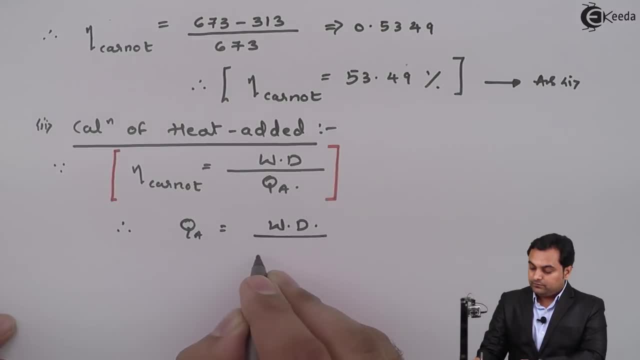 So it will be work done upon the efficiency of Carnot cycle. Now I will put the values. Work done. it is given in the data. It is 130 kJ, So 130 divided by Carnot efficiency. I am going to write the value in the form of number, which is 0.5349.. 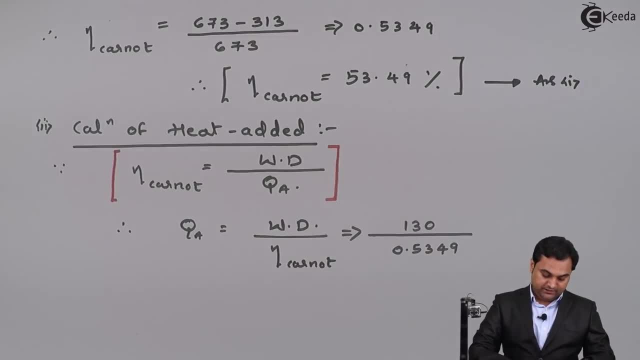 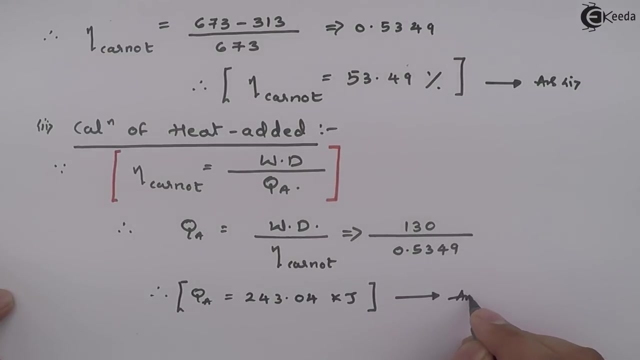 So 0.5349.. So ultimately, My answer is 243.04 kJ. So this much is the heat which is added into the system, And this will be My second answer. So now it is clear that In order to get the work output of 130 kJ, 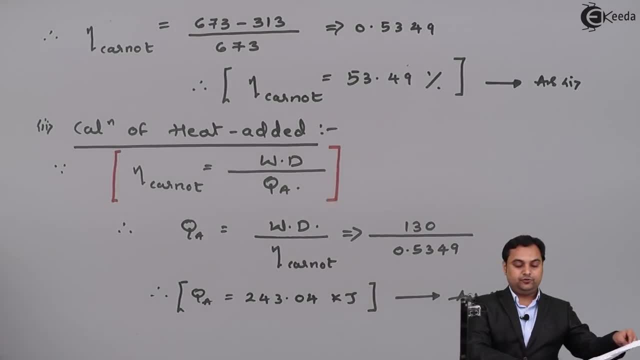 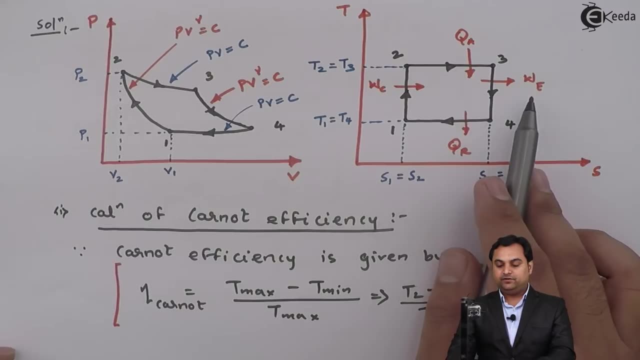 We need to give the heat supply of 243.04 kJ. That I can explain it here, That here we are getting the work output And it is given in the problem that the work output is 130 kJ And for that receiving that 130 kJ. 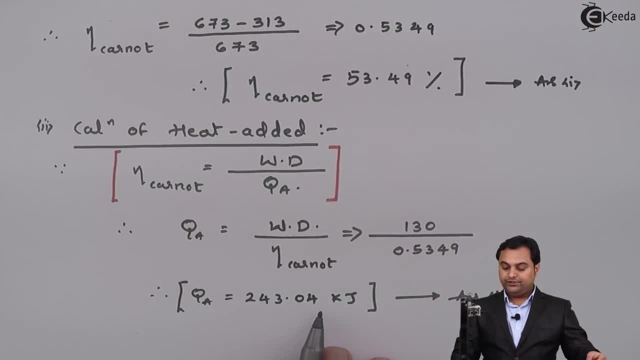 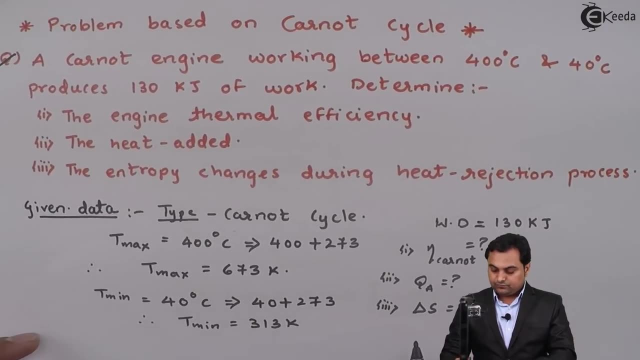 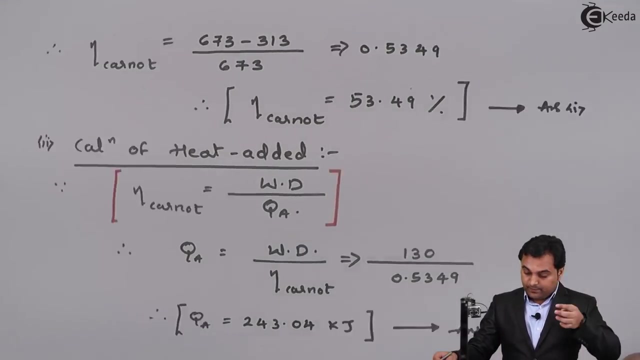 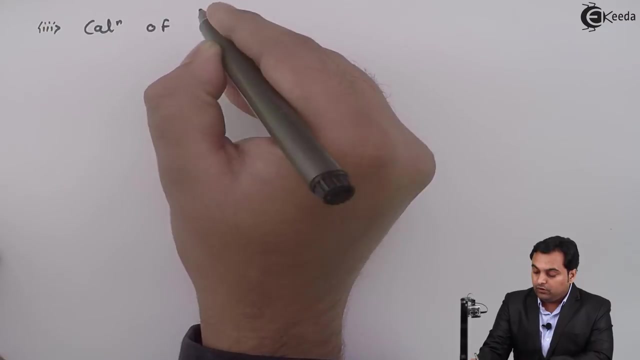 We need to supply a heat of 243.04 kJ. Next, The third question is To calculate the entropy during the heat rejection process, Which is the change in entropy. So I will write down That calculation Of Change in entropy. 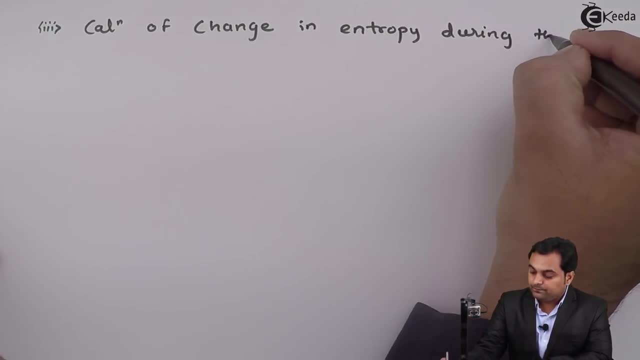 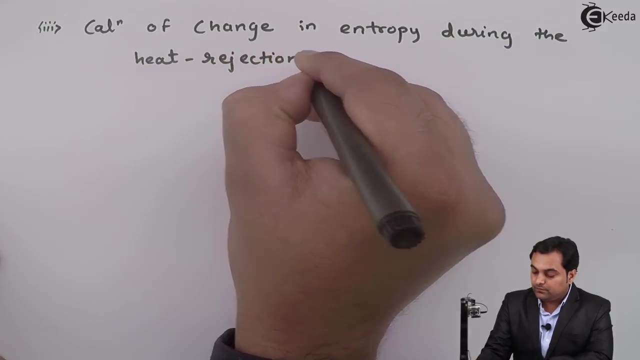 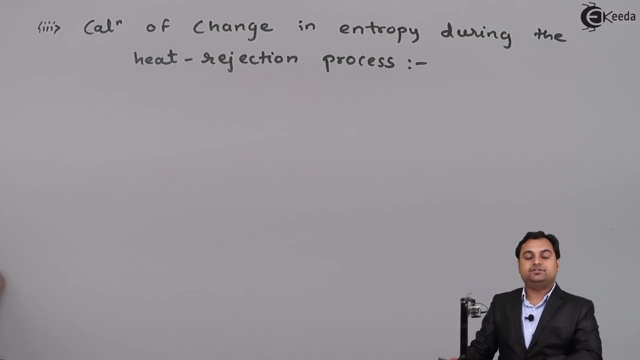 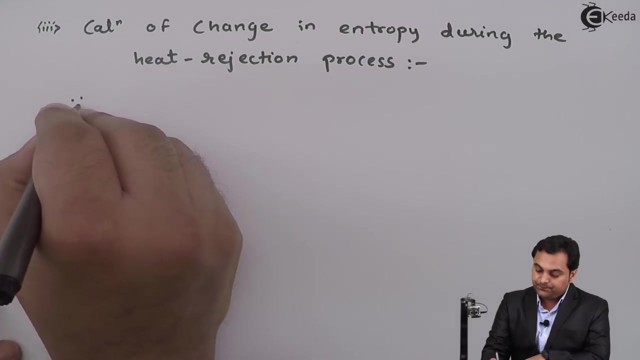 During The heat Rejection Process. Now, How to calculate the change in entropy during the heat rejection process? First is We need to find out how much is the heat rejected. So for that I can say that, since The work done, 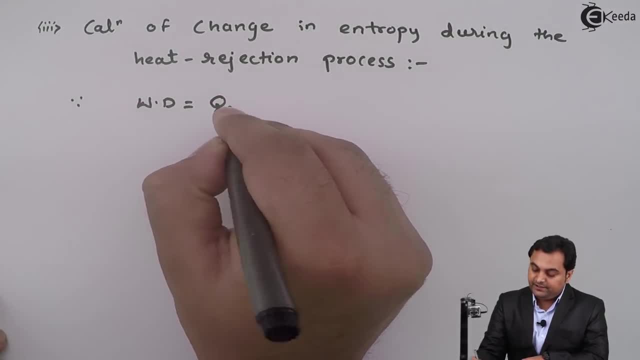 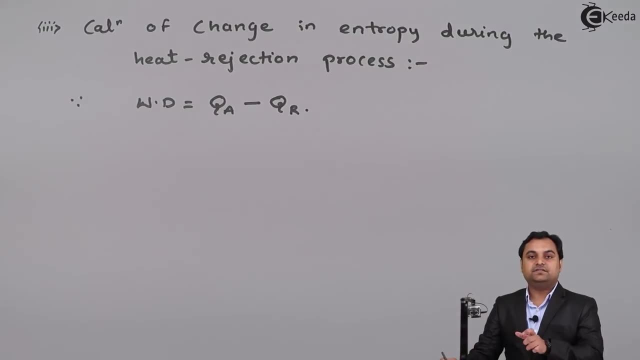 Is equal to Amount of heat added Minus The amount of heat rejected. That is the concept That from the heat supplied, If we subtract the heat rejected, We are going to get how much is the Work which is produced? 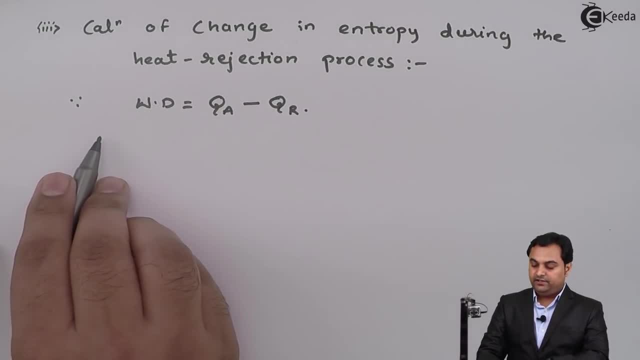 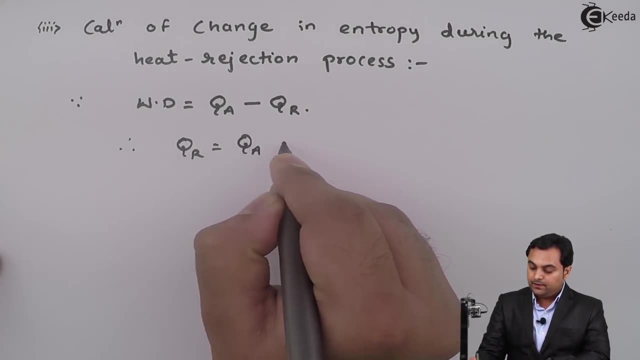 So therefore, if we want heat rejected, I will shift it on to the left hand side And work done will go on right hand side. So therefore, Heat rejected will become QA Minus Work done, So putting the values QR will be. 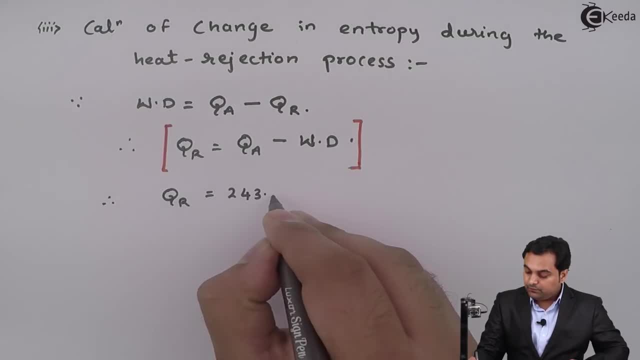 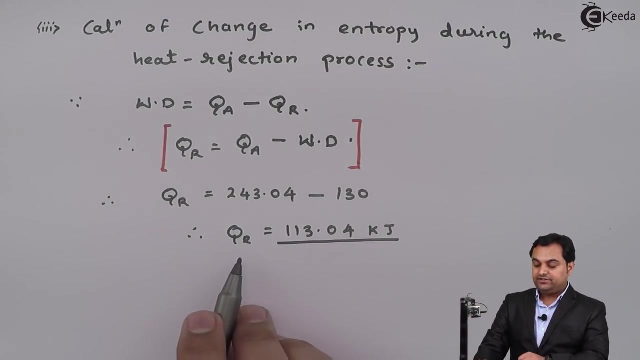 Now heat added was two forty three Point zero four, Minus Work done. It was one thirty. So therefore, heat rejected was found to be Hundred and thirteen Point zero four Kilojoule. Now, after finding the heat rejected, 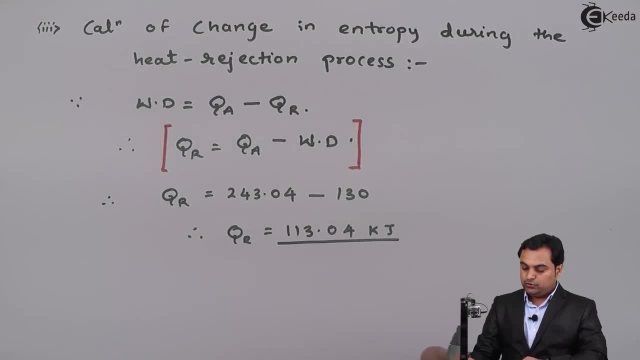 We need to know how much is the change in entropy, So I'll write down. Therefore, Change in entropy Is given by Delta, s Is equal to, And, since I'm finding the change in entropy During the heat rejection process, 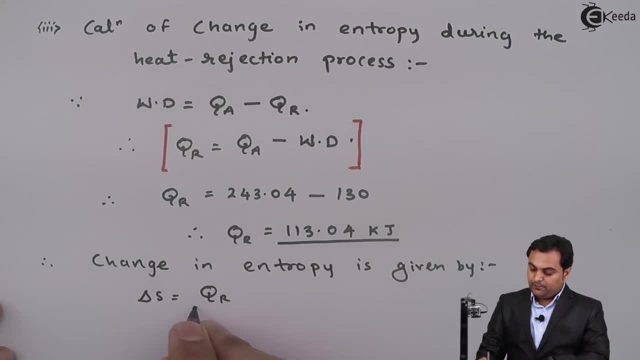 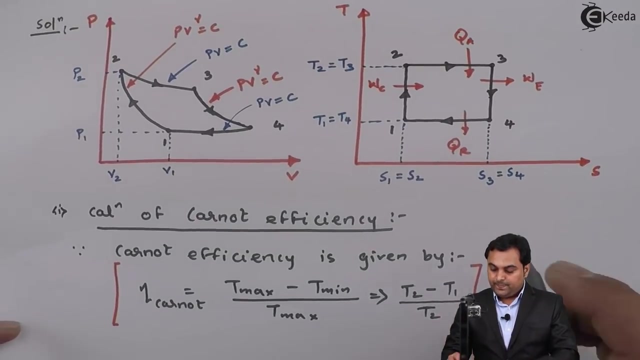 So change in entropy is given by The heat rejected Upon the temperature at which the heat is rejected, And that temperature is Minimum. It is the minimum temperature. If I can explain it On to the T S Diagram, We can see that. 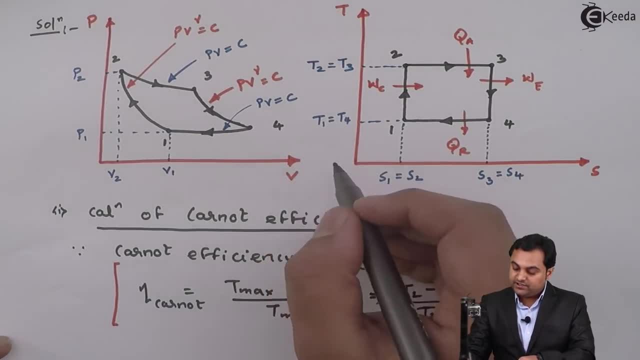 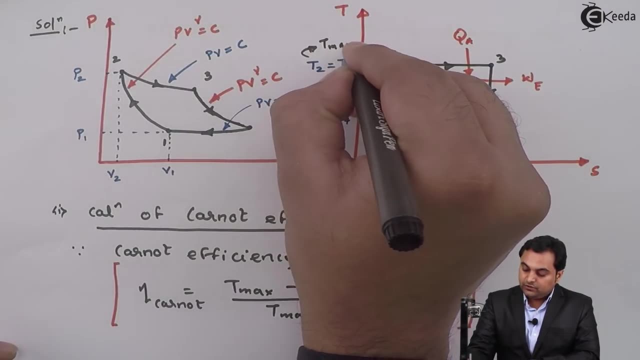 The heat is rejected at: T one is equal to T four And T one is equal to T four. They represent Minimum temperature, Whereas Heat was added at Maximum temperature, T max. So here Heat is rejected at. 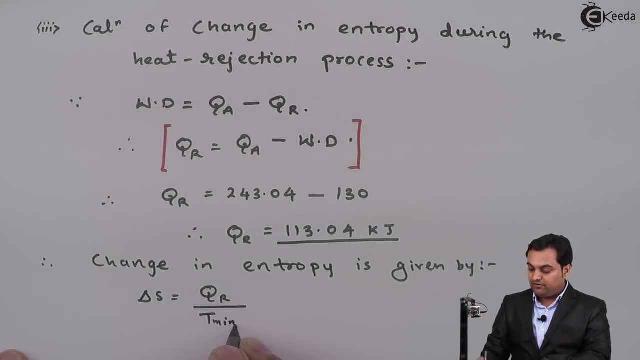 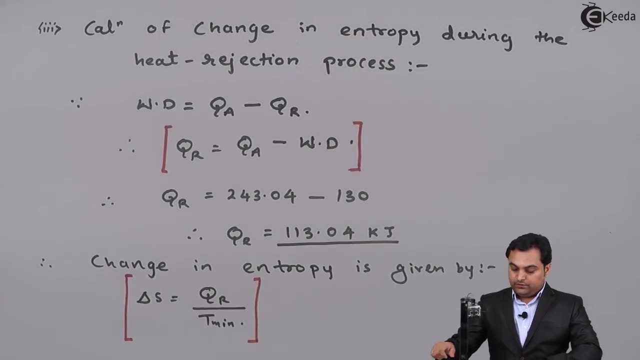 T min. So in the denominator I'll get T min. So this is the formula To calculate the change In entropy, So The temperature at which the heat is rejected. Next, Therefore, I'll find out Delta. 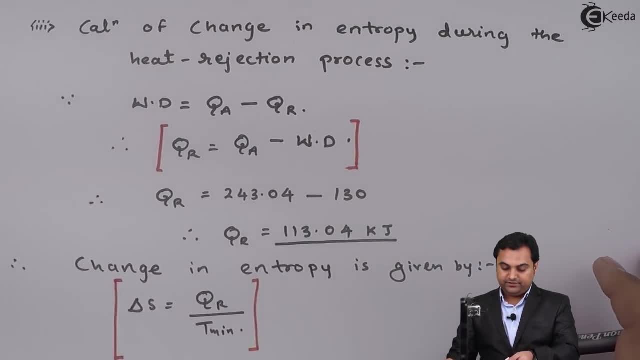 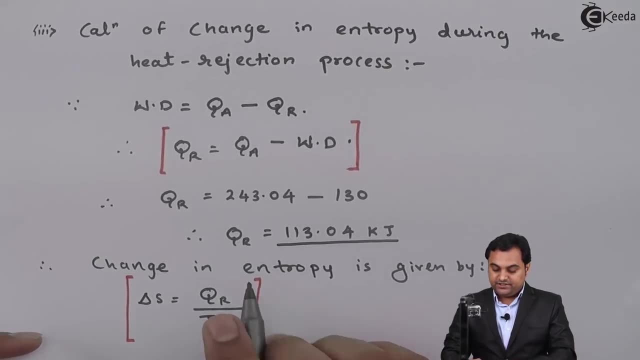 S During the heat rejection process. So Delta S Will be equal to Heat rejected is One hundred and thirteen point Zero four. One hundred and thirteen point Zero four Upon The minimum temperature At T. 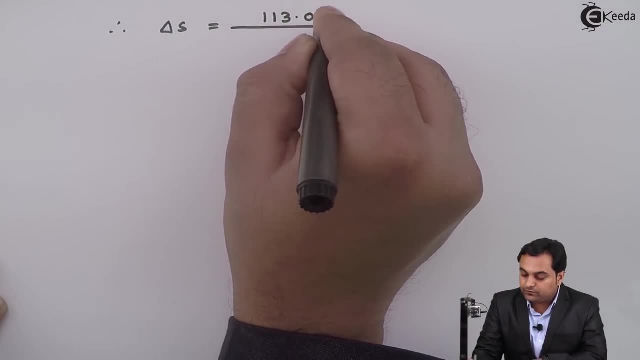 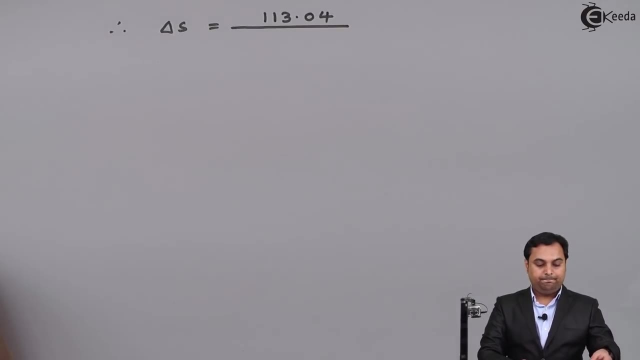 One hundred and thirteen point Zero four. One hundred and thirteen point Zero four Upon The minimum temperature At T min. So the Temperature And minimum temperature Is given in the problem. That is Three hundred and. 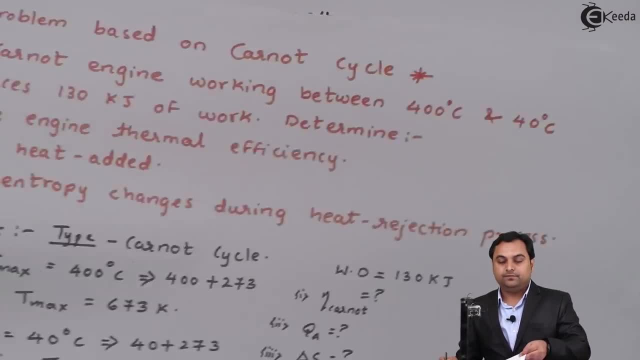 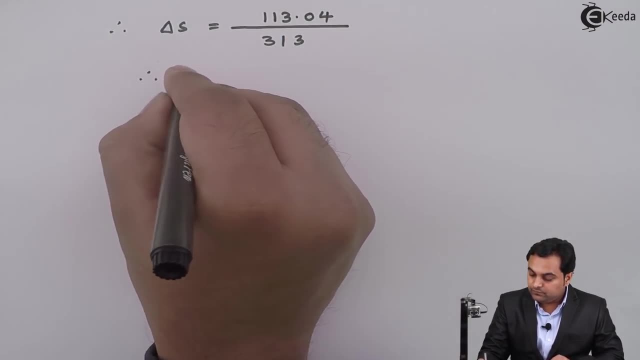 Thirteen Kelvin, So three hundred and Thirteen. Therefore, Delta S Will come out To be Zero point Three six One one. That is The answer. We found out That delta S Will come. 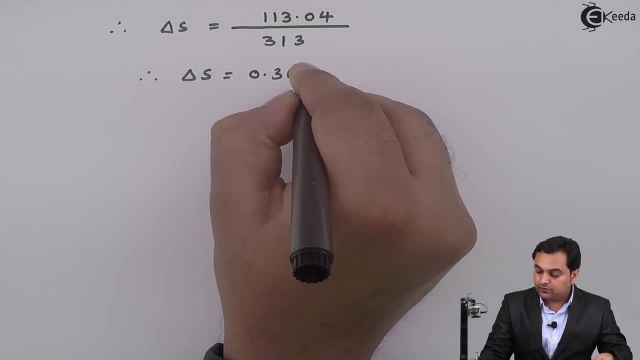 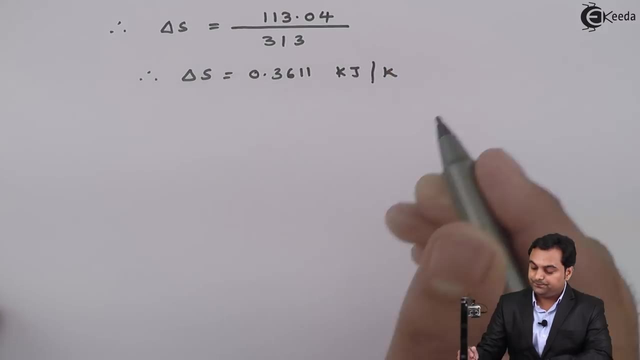 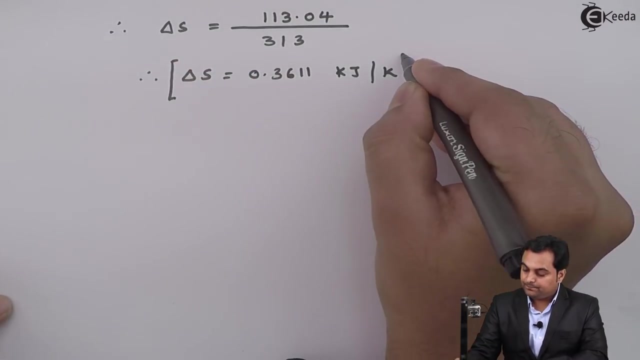 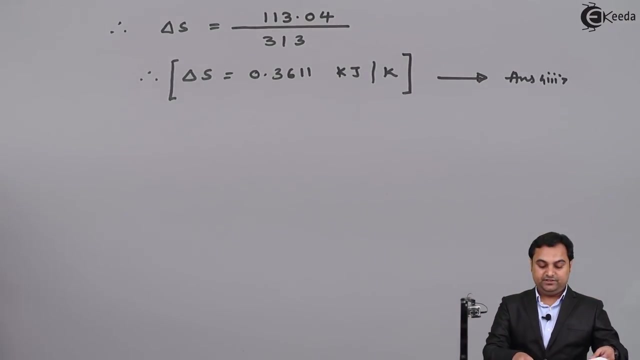 Out To be Zero point Three, six, One, one, That is, are getting and the unit is kilo joule per Kelvin, and this will be the third answer for us. so here, if we see in the question, we were having three unknowns,